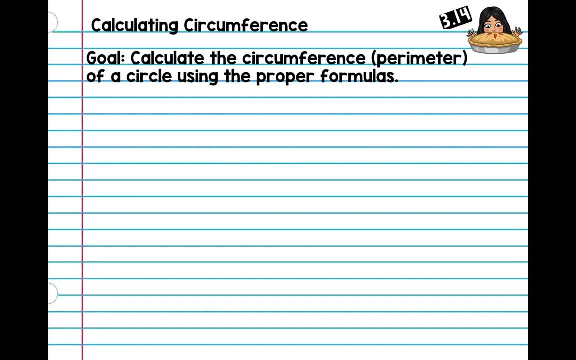 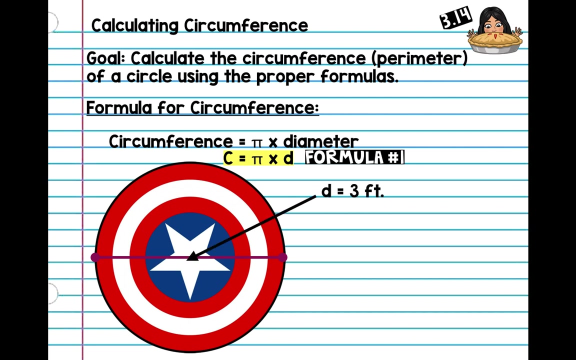 Okay, so grab your notebook and your pencil. Super important that we're writing this down together. Okay, so the formula for circumference is: circumference equals pi times diameter, And that is all. So c equals pi times d. Okay, so this is formula number one. So let's take Captain America's shield. If the diameter across is 3 feet, what is the circumference of its whole shield? 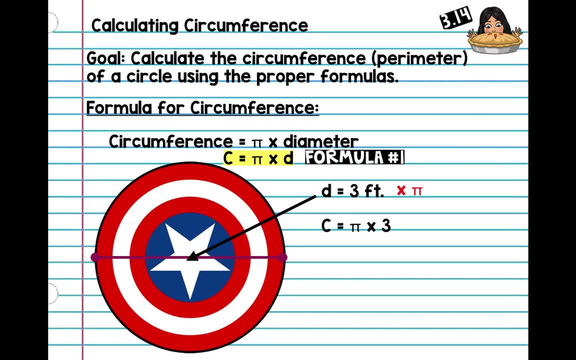 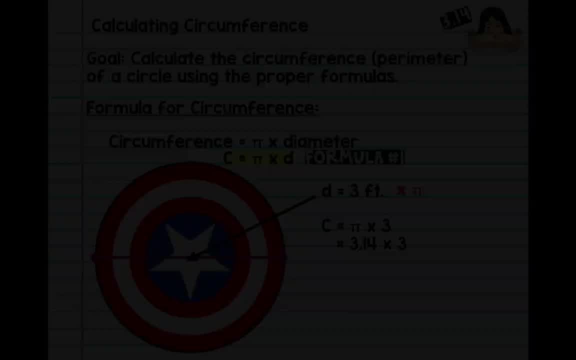 Okay, so let's use the proper formatting. C equals pi times 3,, which equals 3.14 times 3.. And then you're going to grab your calculator, Okay, and we're going to do 3.14 times 3.. 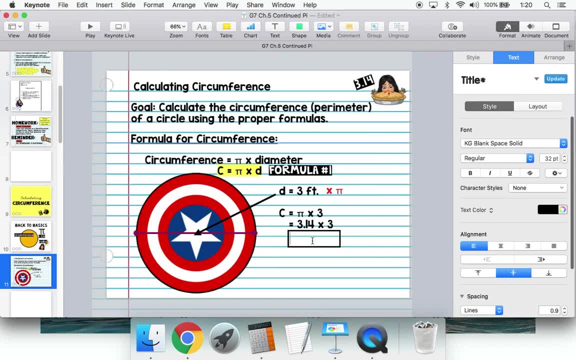 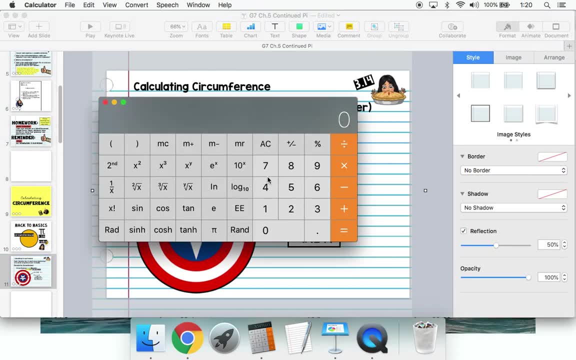 And it equals 9.42.. Okay, so it equals 9.42 feet. Okay, so let me show you using pi. I know you guys don't have your calculators- scientific ones- but it's going to be like this: So 3 times 3 and equals the same thing, 9.42.. Okay. 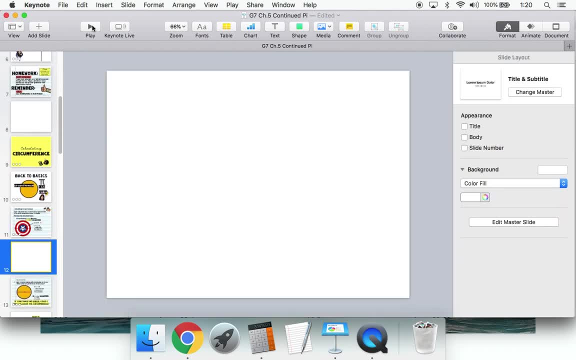 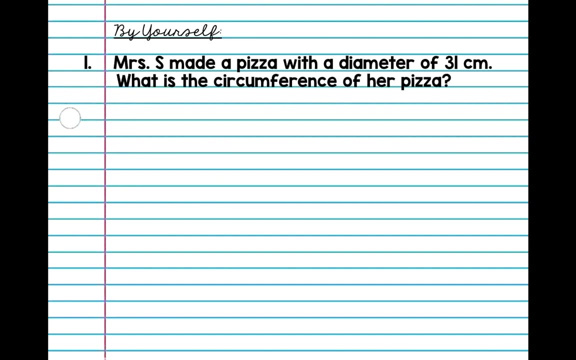 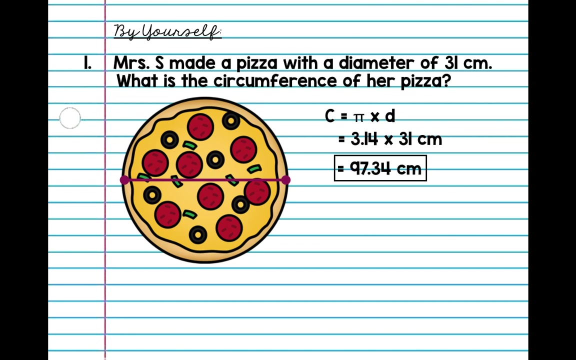 All right, so that was the first part. Good job, guys. All right, so let's go ahead and try one by yourself. Ms S made pizza with a diameter of 31 centimeters. What is the circumference? What is the circumference of her pizza? Go, Okay, All right, so c equals 3.14 times 31.. If you calculated this correctly, it should equal 97.34. 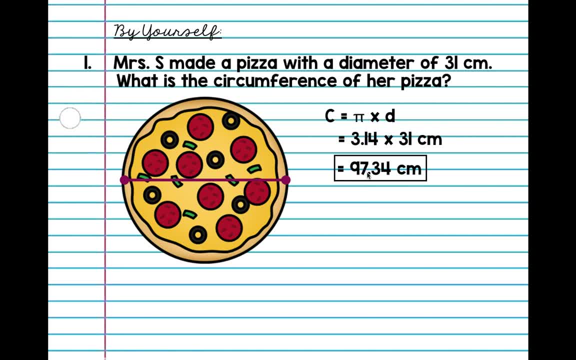 If you used the pi symbol, this would have equaled 97.38.. So on your homework today it's just going to have you know your decimals might be a little different, but just get the one that's closest to your answer. 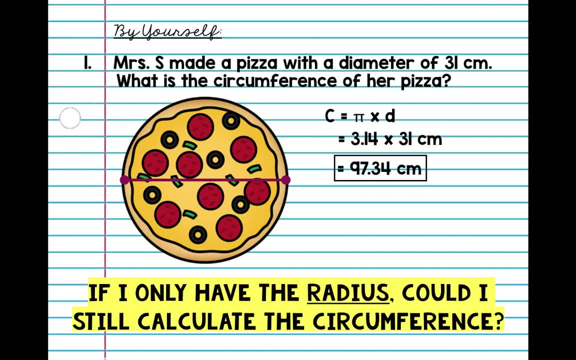 Okay, so Bitcoin Question: If I only had the radius, could I still calculate the circumference? So if I had the circle and they've only given me the radius, would I be able to calculate the perimeter? Okay, so from yesterday, what did you learn about how many radii are in a diameter? Okay, so we learned that we just had to double it Again, multiply it by 2, and it would give us a diameter. So then, second formula is: c equals 3.14. Okay, so we learned that we just had to double it Again, multiply it by 2, and it would give us a diameter. 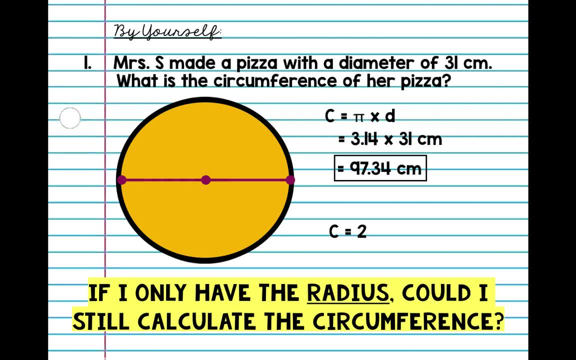 So then second formula is c equals 3.14.. Okay, so we learned that we just had to double it Again, multiply it by 2, and it would give us a diameter. So then second formula is c equals 3.14.. Okay, so we learned that we just had to double it Again, multiply it by 2, and it would give us a diameter. So then second formula is c equals 3.14. 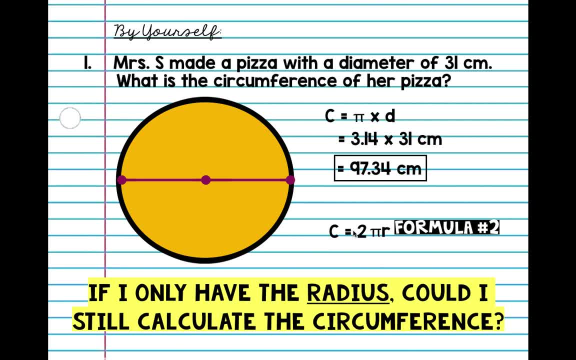 Now, first formula. now, this is stu, which means: how do you do it? What do you do? What do you do? Do you do this thing? It goes into this p-shaped circle formula. so just memorize: c equals 2 pi r, and that's all you have to remember, okay? so let's. 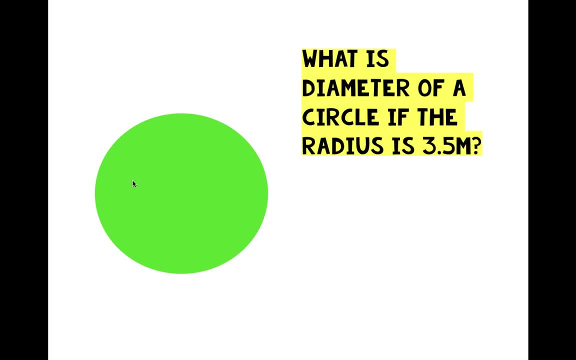 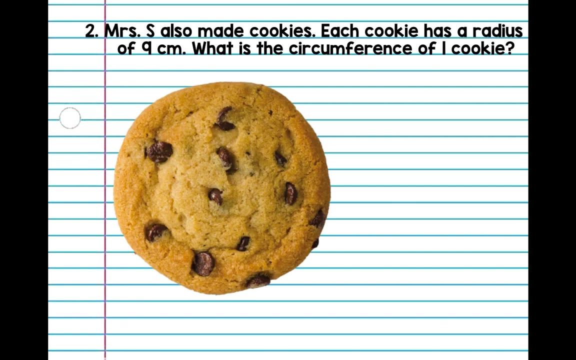 review. so what is the diameter of a circle diameter if the radius is 3.5 meters? okay, so you're going to go 3.5 times 2, which equals 7. all right, and that's what we're going to be doing. so why don't you try this problem by yourself? um miss s also made cookies each. 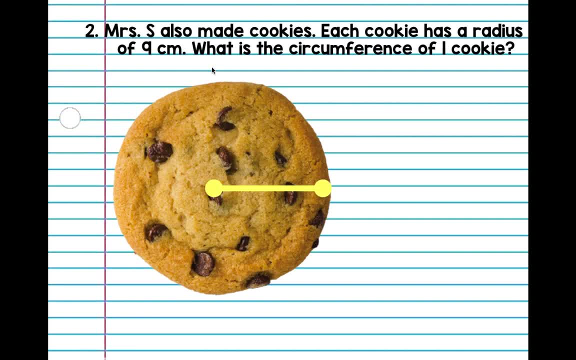 cookie has a radius of 9. okay, what is the circumference of one cookie? okay, so go ahead and use your proper formula: c equals 2 pi r. okay, all right. so let's go. we have 2 times 3.14, times 9, and you can just do whichever one you want to do first, and if you calculate it correctly, it should. 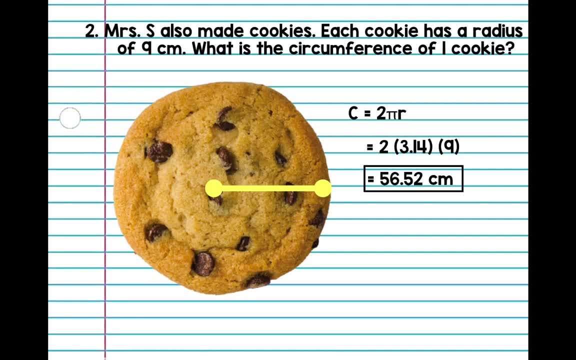 be 56.52. we just estimate the radius of the circle diameter and then we're going to go 3.5 times 2 and estimate it's going to be about 57 centimeters. so my cookie has a circumference of 57 centimeters. 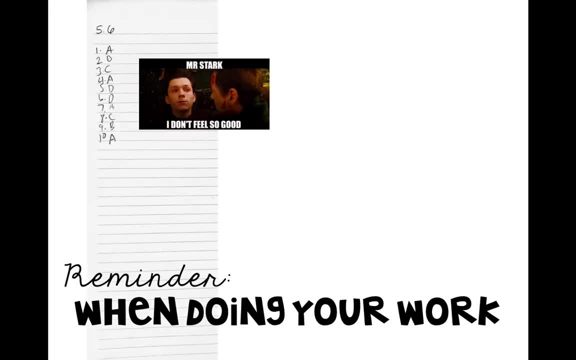 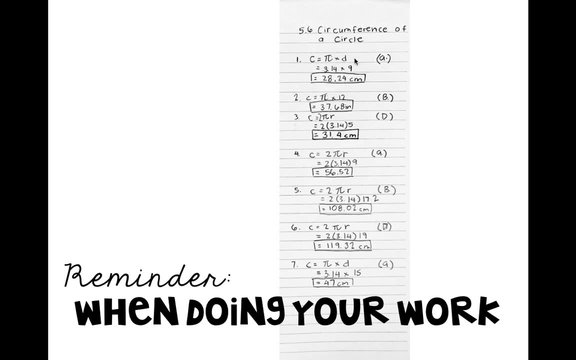 all right. so great job today, guys, when you're doing your homework again, show your work. it wouldn't feel so good if you did this. um, if you look here, because you guys are using a calculator, which is super easy. just make sure your formatting is proper. okay, it's 2 pi r, all right, so let me. 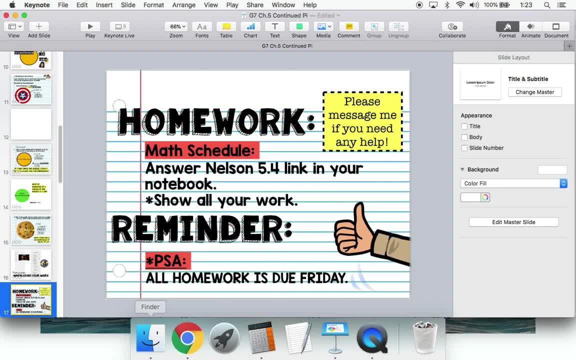 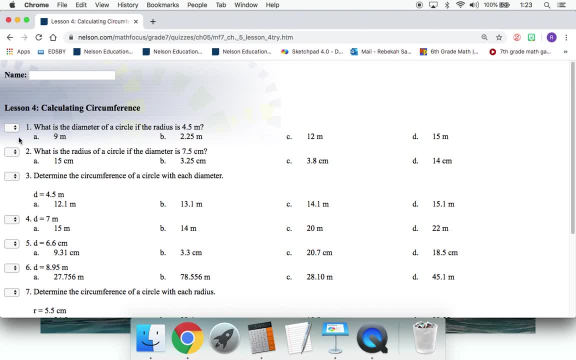 show you your homework is going to be the 5.4 link, so it looks like this: um, what is the diameter if the radius is 4.5? so you just multiply that by 2, which one's the answer. okay, it's going to ask you for the circumference of the diameter. um, i mean,